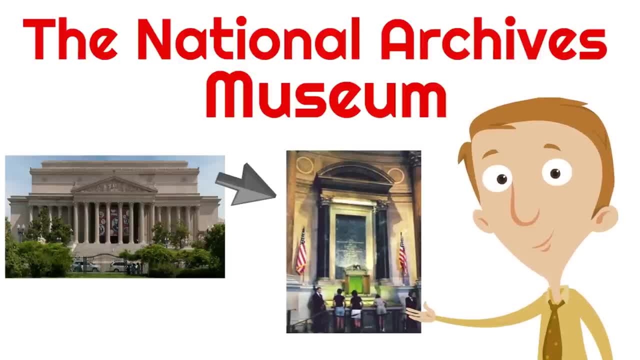 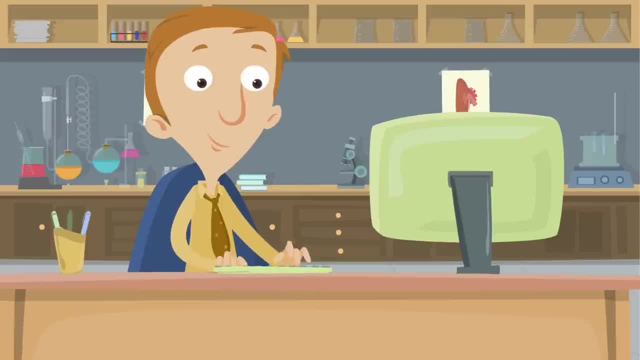 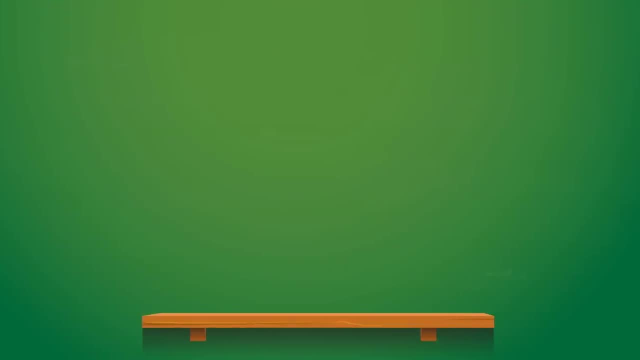 started the United States of America. But let's not get ahead of ourselves. We want to give you the full story of the Declaration of Independence, so you can see why it is so special. We mentioned that the Declaration of Independence was signed in 1776.. To understand the Declaration, 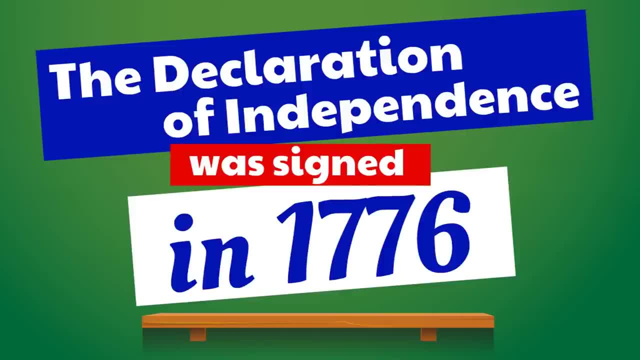 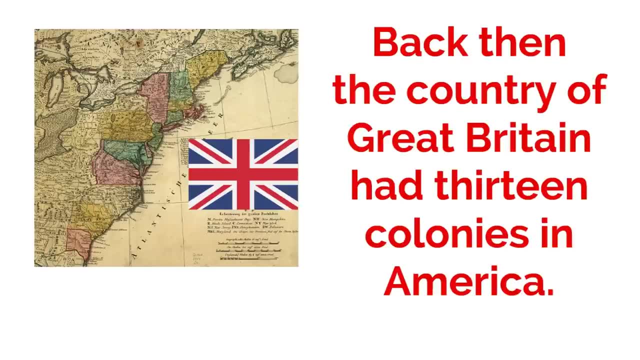 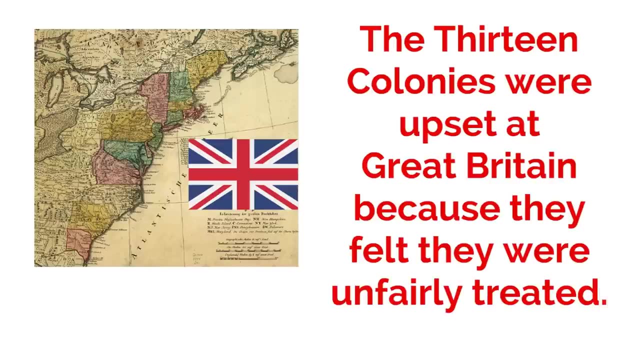 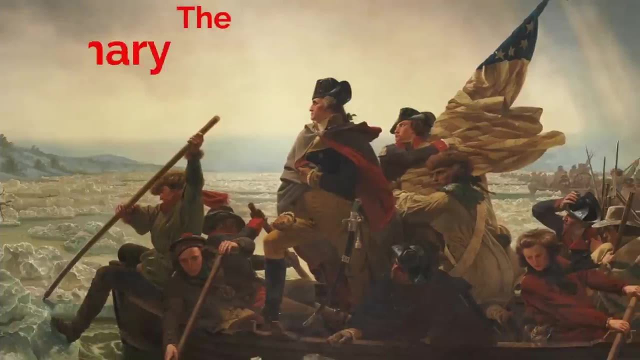 of Independence. we have to know what was going on at that time. Back then the country of Great Britain had 13,000 people. The 13 colonies were upset at Great Britain because they felt they were unfairly treated. One thing led to another and the 13 colonies went to war with Great Britain in a war called. 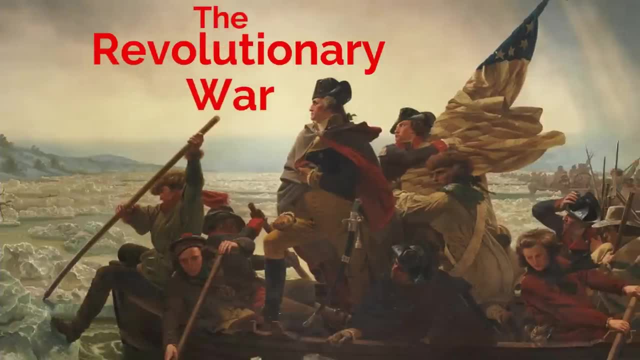 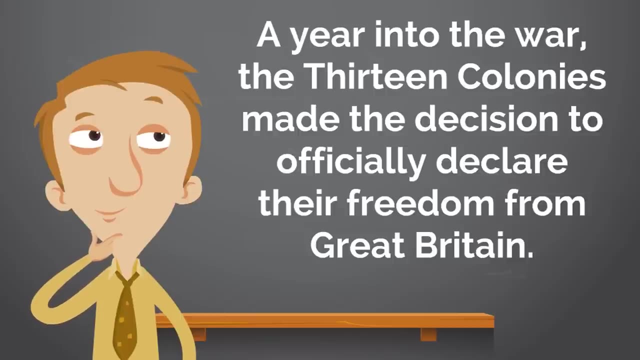 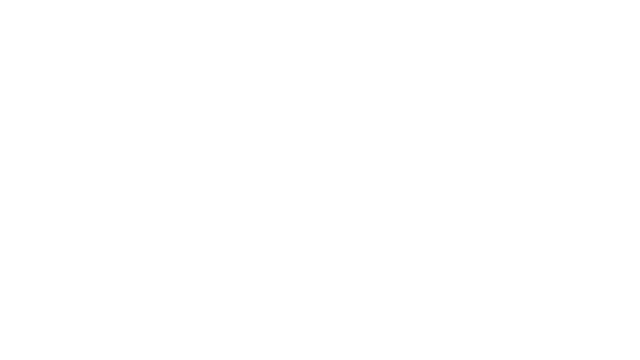 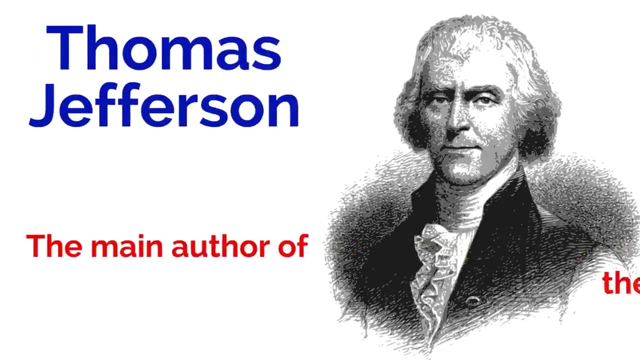 the Revolutionary War. A year into the war, the 13 colonies made the decision to officially declare their freedom from Great Britain. So they got help from this guy, a gentleman named Thomas Jefferson. Have you heard of him? Thomas Jefferson was the main author of the Declaration of Independence and it was his. 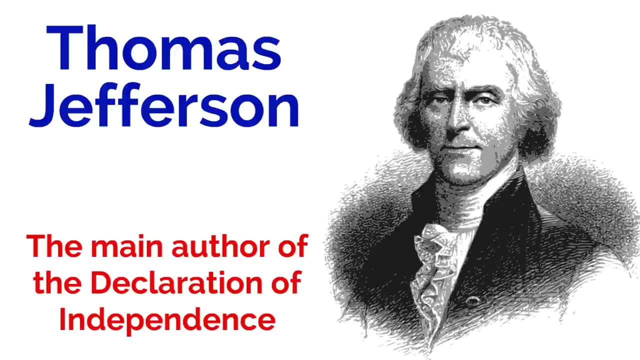 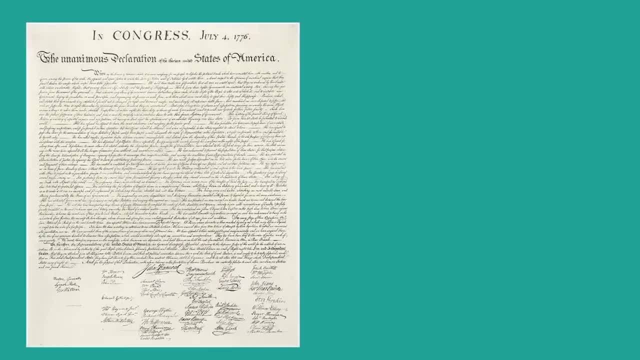 job to put to words exactly why they were declaring independence, And that's what the Declaration of Independence does. The Declaration of Independence explains why the 13 colonies were so important to Great Britain. The Declaration of Independence explains why the 13 colonies were so important to Great 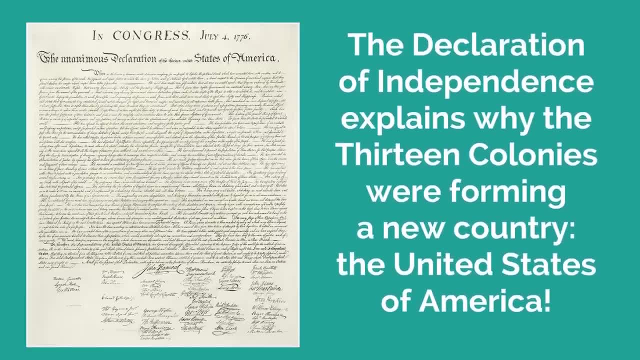 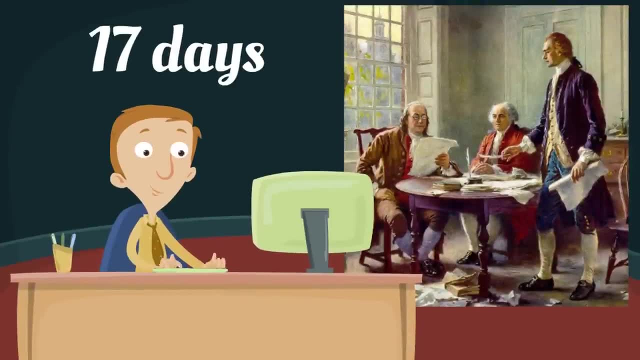 Britain. We want to present to you the content of the Declaration of Independence's language. The Declaration of Independence states that the three individual nations were consummodern and at the same time civilized. The Declaration of Independence states that the 15 nations would haveky inherit their 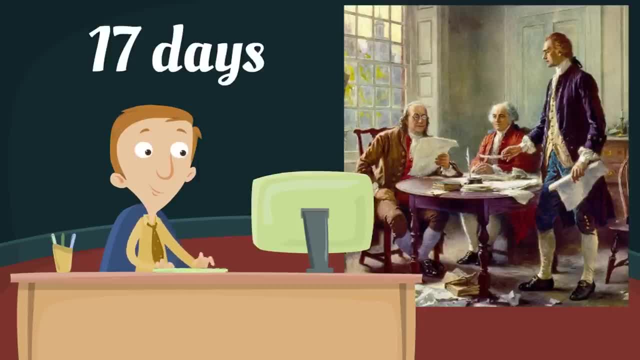 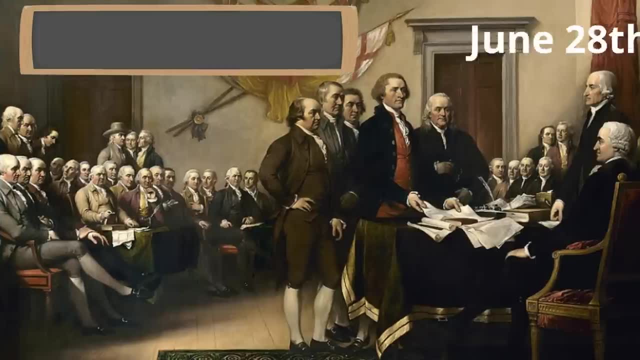 throne, while it沒關係 them with another nation and kissing. Consider this: The Declaration of Independence already dated thousands of years before 16 at the time. And catch this: on June 28, 1776,, Thomas Jefferson and the committee shared the document with the Second Continental Congress in Independence Hall. 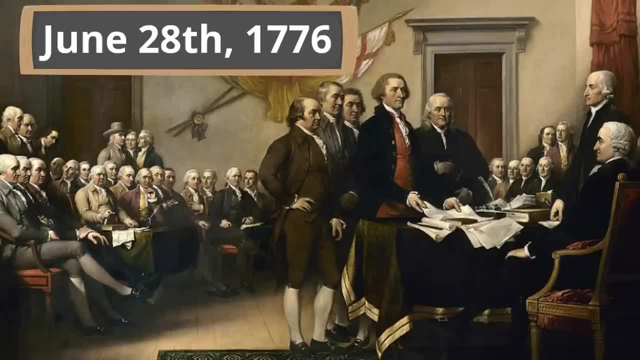 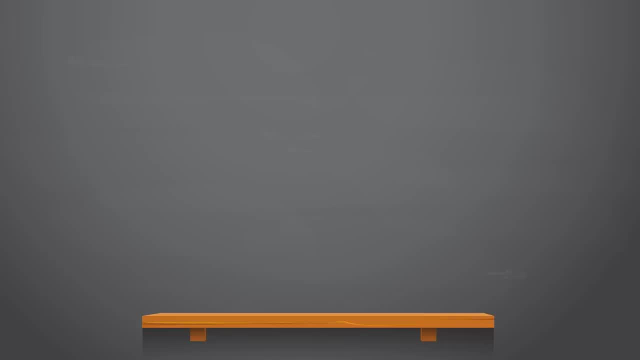 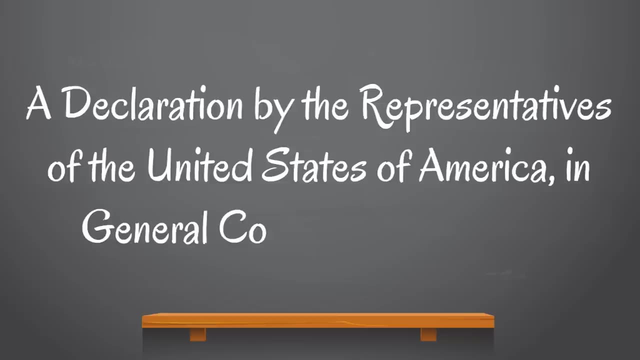 And- interesting fact- when they shared it with the Second Continental Congress, it wasn't actually called the Declaration of Independence. They originally called it a Declaration by the Representatives of the United States of America in General Congress Assembled. Wow, long title, That's a long title. I'm glad it was shortened right. 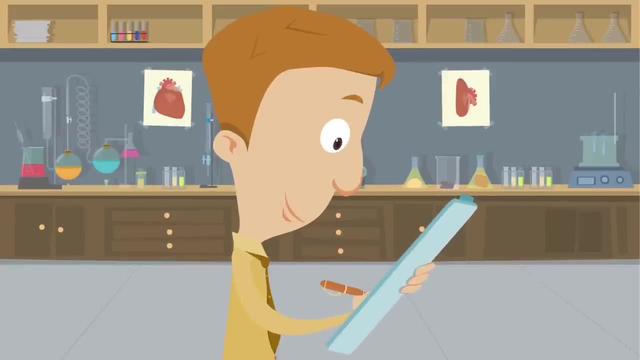 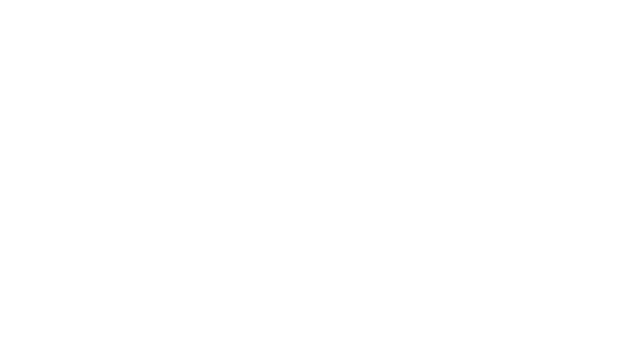 Once they had the document, Congress made changes. They shortened the document itself and the document became known as simply the Declaration of Independence. Then the big day came: On July 4, 1776, Congress voted for the Declaration of Independence. The date was written on the Declaration of Independence and, even though it was not signed by everyone right away, it became official. that day, The first person to sign the Declaration of Independence was a guy by the name of John Hancock. It made sense. He was the president of the Second Continental Congress. 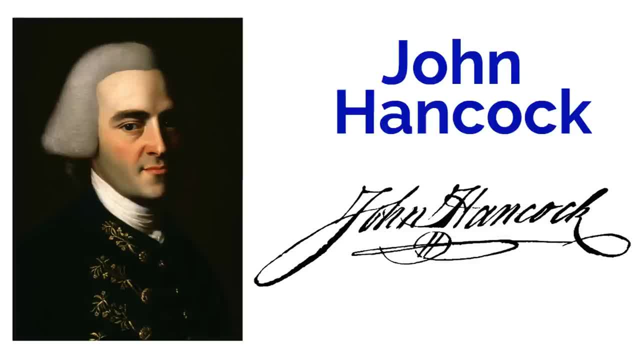 He is famous for his signature on the Declaration of Independence because he wrote his signature with such big letters. You can see his signature here. Plus, this is a super cool signature. Do you see this H down here? That's really cool. 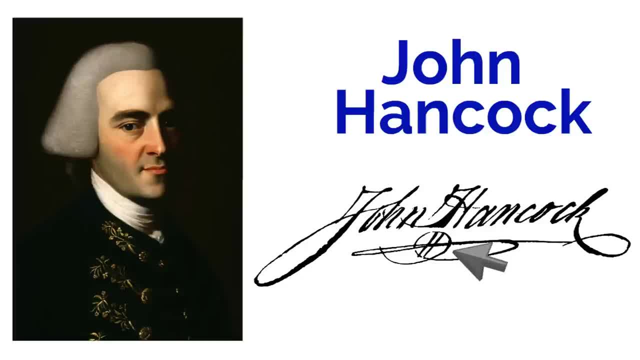 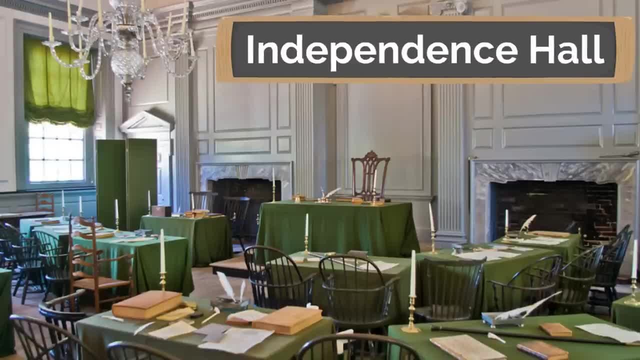 There's like an H and a loop and wow, That's awesome. That is so cool. Did you know you could visit Independence Hall today? Independence Hall, remember, is the place where Thomas Jefferson and the committee shared the Declaration of Independence with the Second Continental Congress. 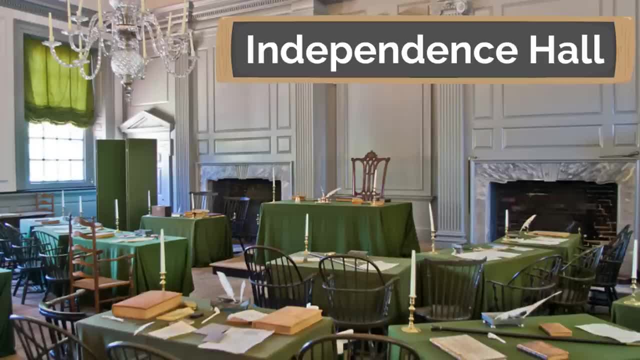 It's where the Declaration of Independence was voted on and it's where the Declaration of Independence was signed by John Hancock and others. So just visit Independence Hall in Philadelphia if you want to see these cool green tablecloths in person. 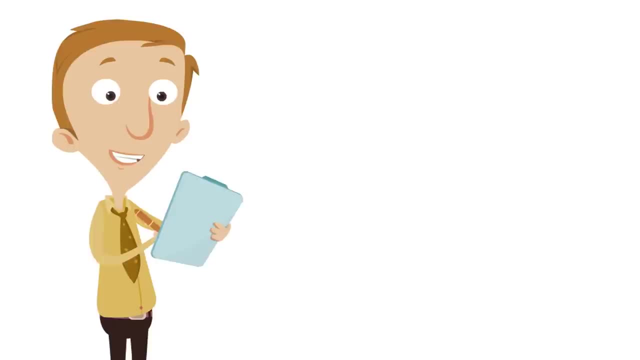 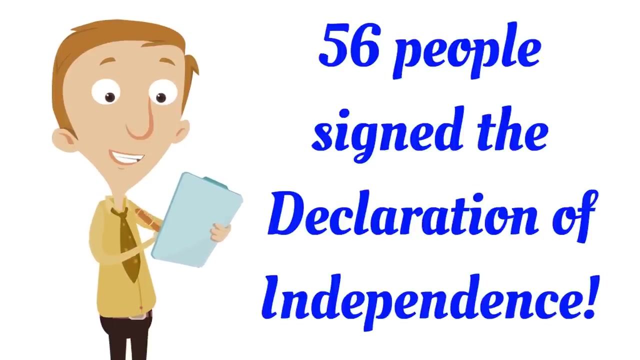 So the Declaration of Independence was signed, but it wasn't signed all at once. not at one time- And this is interesting- 56 people signed the Declaration of Independence. Isn't that incredible? 56 people Share that with somebody right now.